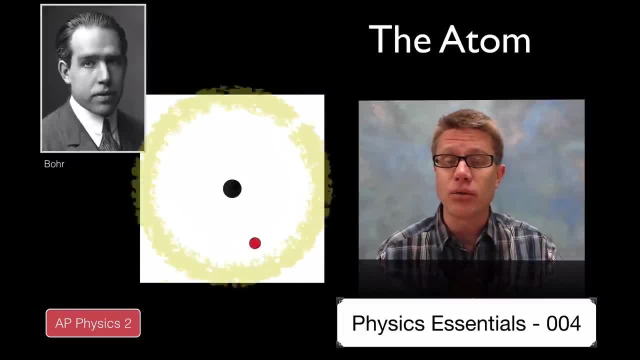 He also knew that as it gives off radiation, the wavelength of that radiation is going to vary, And as it varies we are going to get this nice smooth spectrum Spectrum of electromagnetic radiation given off by high energy atoms. But when we started to look into space, what? 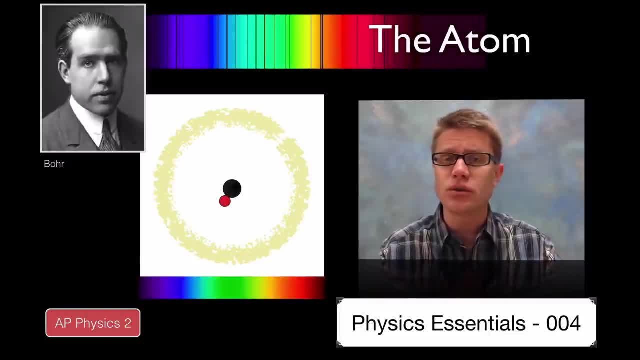 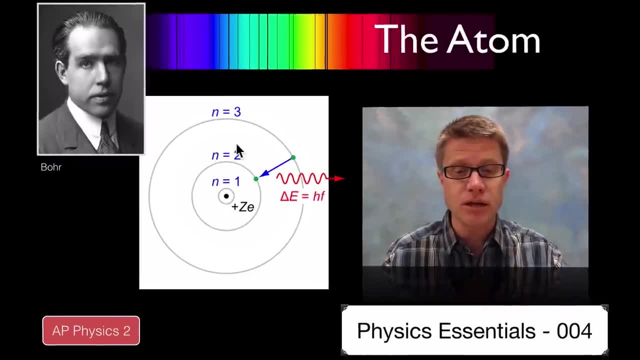 we found is that light wasn't smooth. It had these discrete units within it, And so that spectra had to be described, And Bohr's model helped to do that. And so, if you think of it like this- and this works, for hydrogen is what the Bohr model is built on- You have 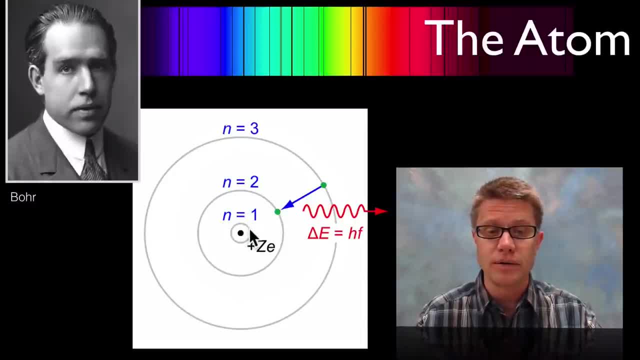 these energy levels, And so an electron can be in energy level 1.. And so an electron can be in energy level 2.. And so an electron can be in energy level 3.. And so an electron can be in energy level 1., Energy level 2., Energy level 3., But it can never be found in the 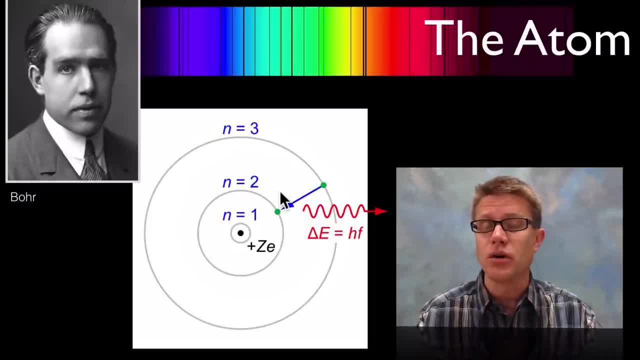 middle. It is quantized. It has to be in one of those levels or another level. And so how does it move between levels? Well, if it absorbs energy from a photon electromagnetic radiation, for example, it will jump to a higher level, And as it moves down it is going to emit those. 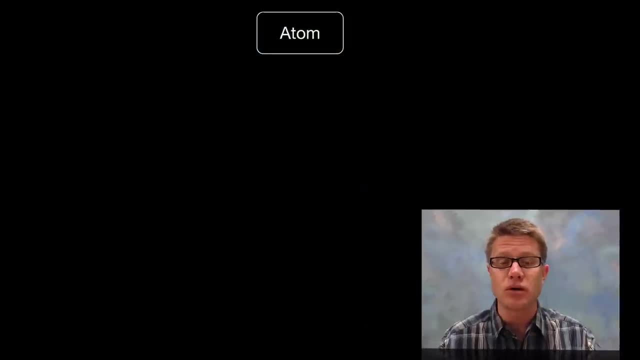 photons And that helped to describe what we were seeing in the spectra, And so that improved our model. So we now had the cloud that had the electrons in it And as it moved down it was going to emit those photons, And that helped to describe what we were seeing. 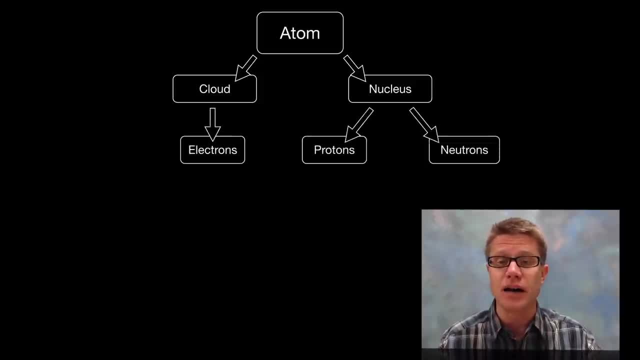 in the spectra And as it moved down it was going to emit those electrons in it, And then the nucleus, And so we found these negative electrons in the cloud. And then protons and neutrons were found in the nucleus And in a neutral atom. the number of protons and 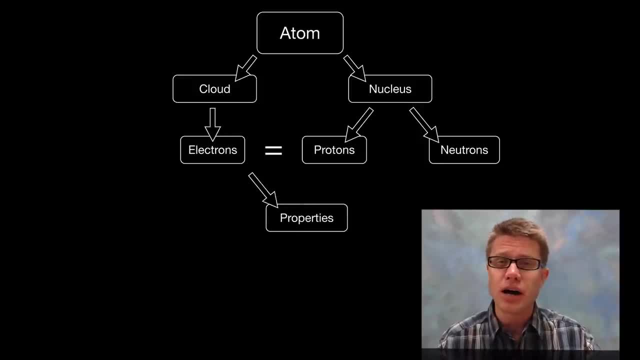 electrons are going to be equal And the electrons tell us a lot about the properties of that atom. In fact the whole periodic table is built on the electrons, Electrons especially, we have in these outer levels. Now the Bohr model helps us explain what those electrons. 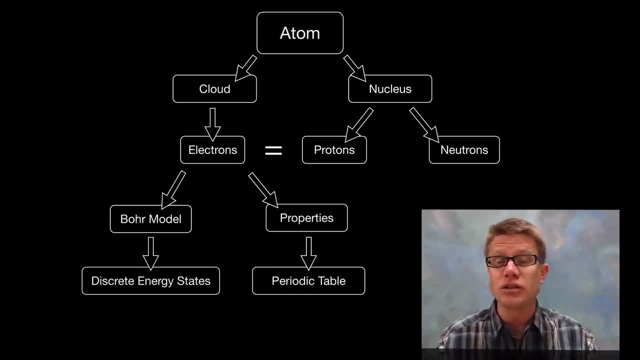 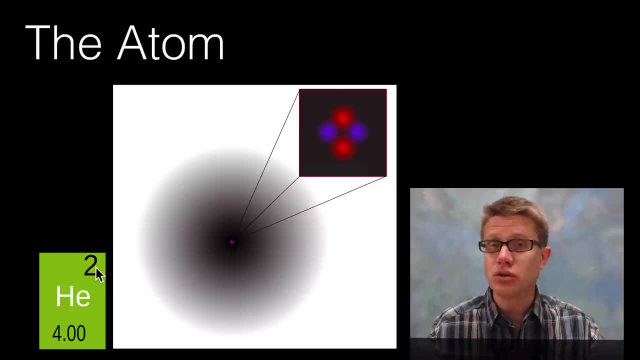 are doing and how they are moving. They move into these discrete energy states, And that helps us to explain the spectra. And so if you look at any kind of an atom on the periodic table, the atomic number 2 tells us the number of protons we have. And so we are going to. 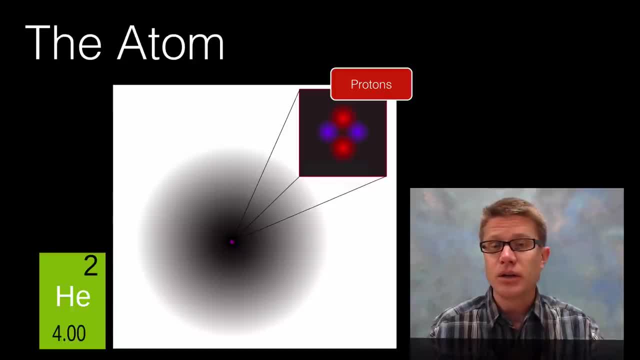 have these positive protons that are going to be found in the nucleus. We can kind of figure out how many neutrons, roughly, we are going to have in an average atom by taking the mass number subtracting the atomic number, And so we would know in helium, for example, 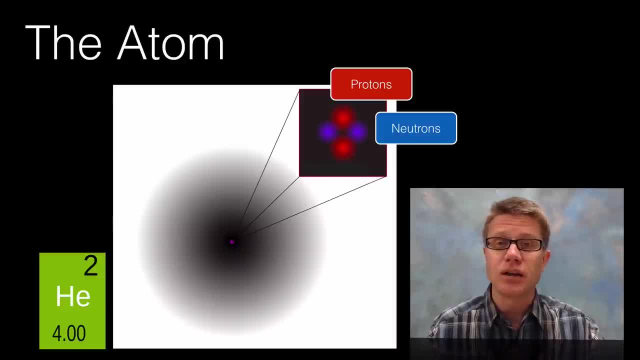 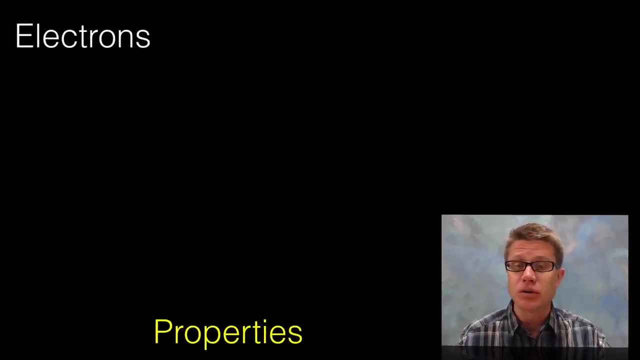 that we are going to have two neutrons. Now, since the number of protons and electrons are the same in a neutral atom, we can figure out that we have got these electrons And these electrons moving around the outside And the number of electrons that we have out. 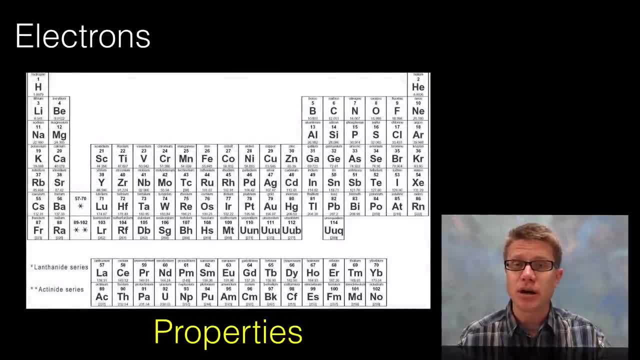 there tell us a lot about the properties of the atom, And so if you look at the periodic table, this whole thing is essentially built on the number of electrons that we have, Because that tells us a lot about the properties, And so if you look right here we will find. 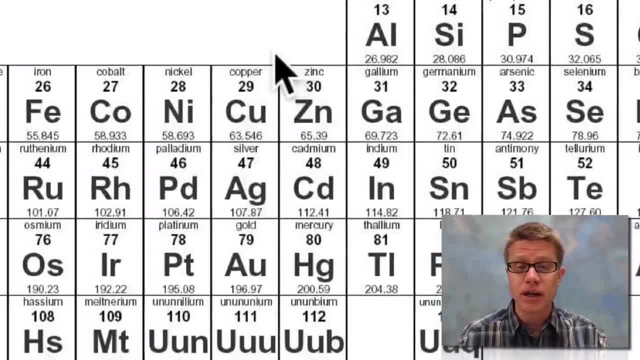 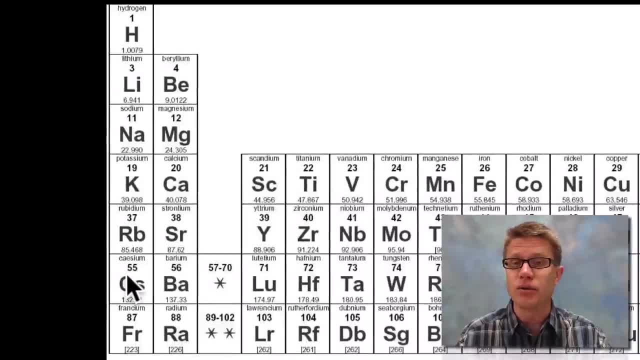 copper, silver and gold, which are all very similar, are in the same column And that essentially says that they have similar outer level electrons. Or, if we look in the first column, all of these are highly reactive. All the noble gases are neutral. All of these 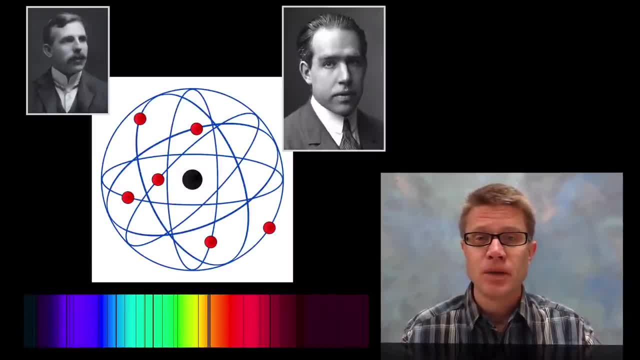 are not, And so the properties of atoms are built on those electrons. But there were problems with this planetary model: Electrons were not orbiting like planets, They were actually jumping between orbits, according to Niels Bohr, And so they did not just move back and 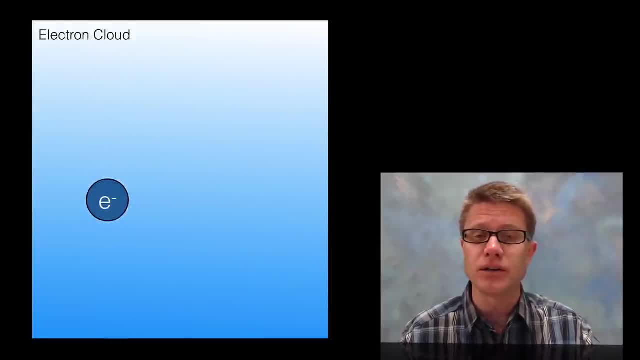 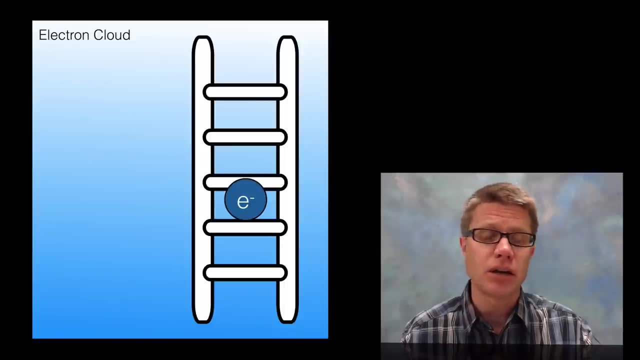 forth on all these infinite number of orbits around the nucleus, giving off a smooth amount of spectrum, Almost like a ladder, That an electron could be here, but it could also be here And it could never be found in the middle. We call that being quantized, If you. 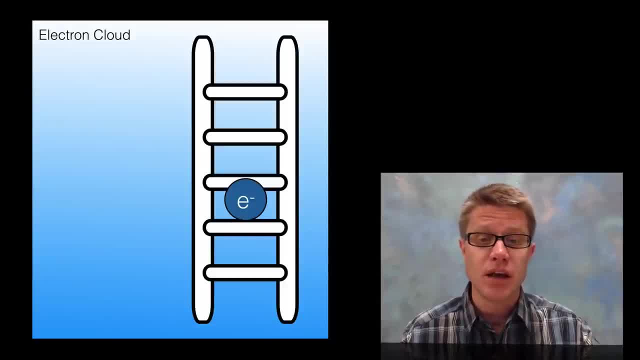 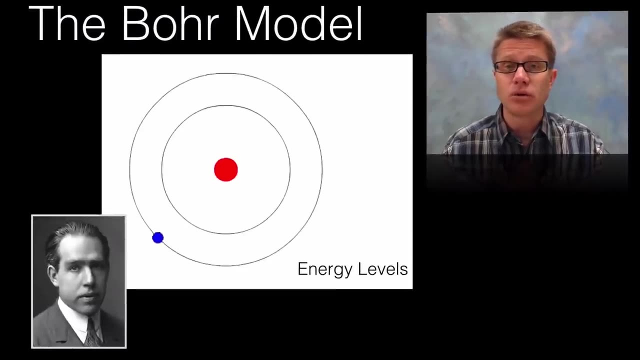 look at the electron: it has to be in a specific unit to exist. Now, how do you move an electron to a farther level? Well, you have to put a little bit of energy into it. So if we add a lot of energy, we could jump it up to this energy level And as it falls back down, it's going to release a certain amount of energy, And so this is a visual or a model of what the Bohr model might look like. And so, as it orbits around the center, if it receives a photon, it jumps to a higher level. If it gives off an equal photon, it will drop down. 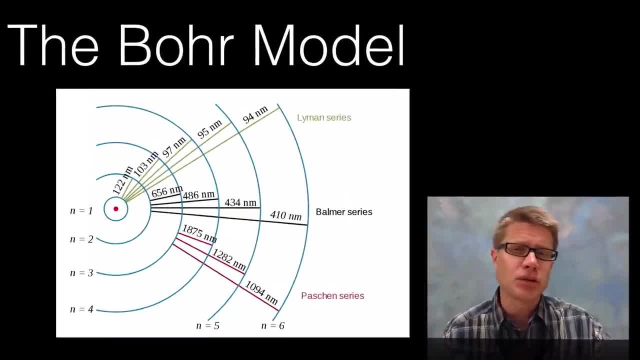 to a lower level, And so it's only a matter of how much energy it can take to get to the center. So it's only existing in these quantized orbits, And this helped to explain spectra, Because before the model was discovered or was put forth, people had started discovering. 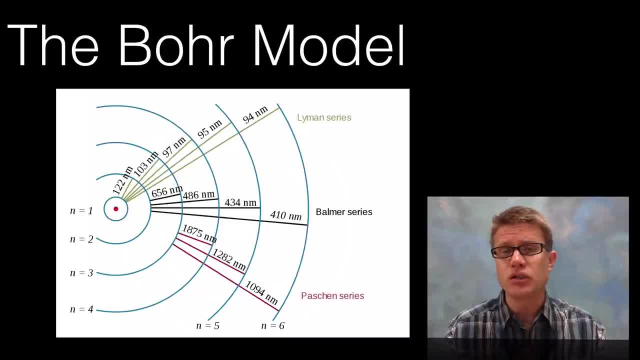 spectra. They were looking into space not with just a prism, but a spectroscope, So they were splitting the light into all of its different wavelengths And they were starting to see these lines. So when you're looking at the sun, for example, which is mostly hydrogen, 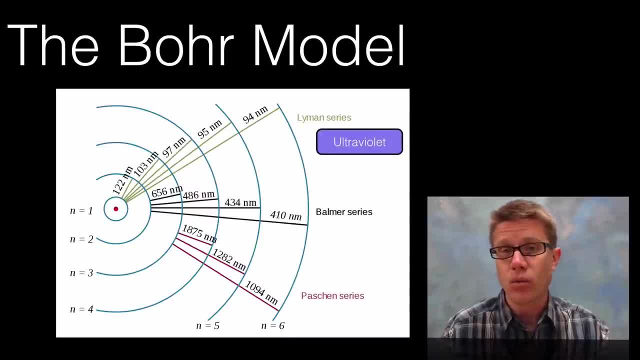 we saw these different series. So the Lyman series was developed by one scientist And he was using spectroscopy And he came up with an equation that explained what was going on. But you couldn't see this spectra because it was into ultraviolet. We also saw 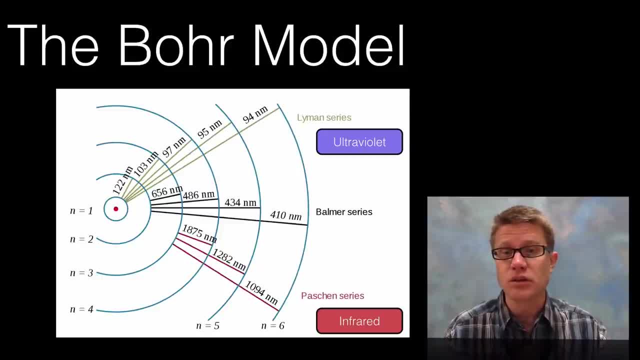 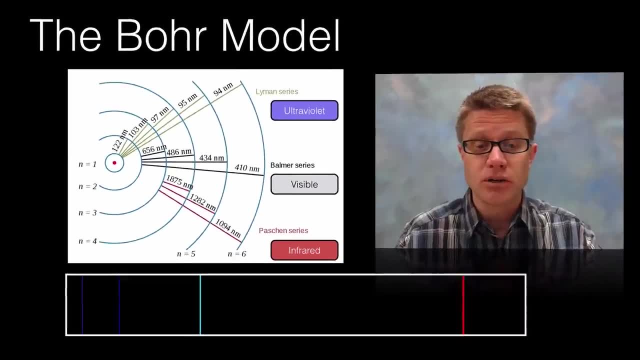 the passion series that was showing the similar relationship, But this was in the infrared And the Balmer series was seeing the same thing, And so what really he was explaining- let's throw the Balmer series up here- is that they were seeing these discrete units. 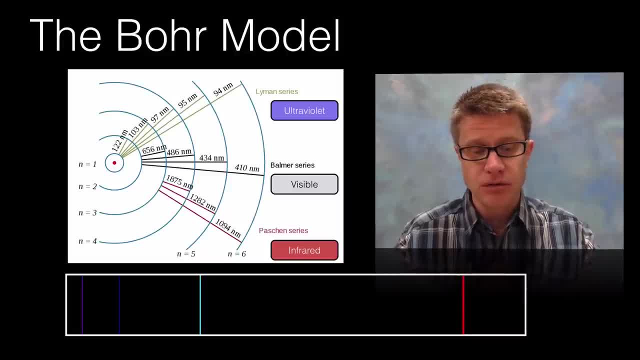 of light, And so where was that light coming from? If you look at hydrogen, well, you can see here, as we move from this energy level 2 up to energy level 3, it requires a certain amount of energy And as the electron falls back down, it's going to give off that energy. 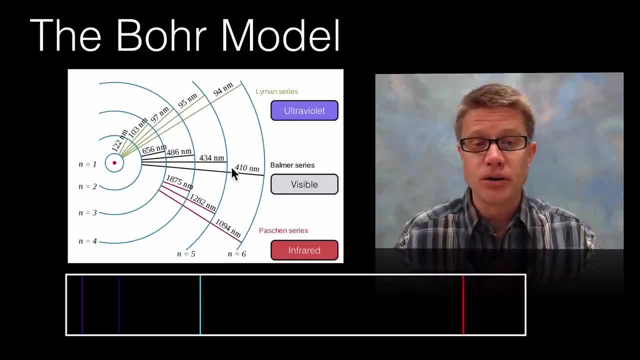 It's going to give off that light, And so the Bohr model predicted what these numbers were, And they fit perfectly with the numbers that we were seeing in the spectra, And so, again, this only works for hydrogen, And so it's a good step model, or it's a good model. 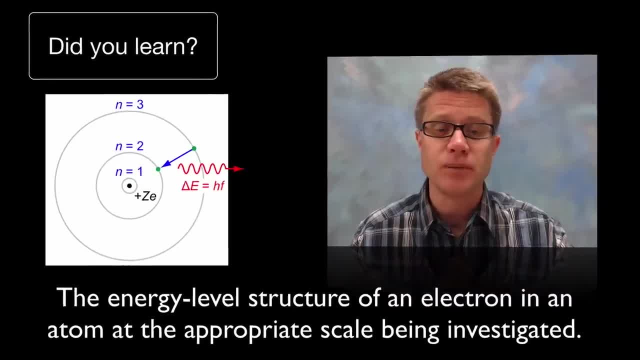 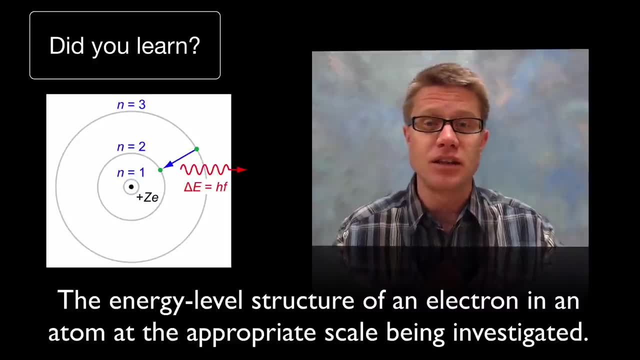 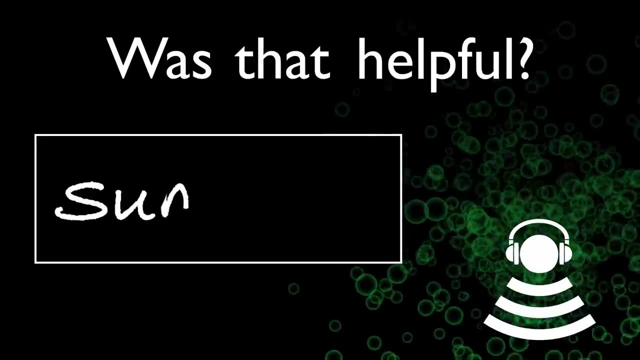 to get you started on understanding how the atom is really put together: structure. But did you learn the energy level structure of an electron in an atom at the appropriate scale being investigated? In this case it is at these energy levels in hydrogen atom. I hope so. That is the Bohr model And I hope that was helpful.